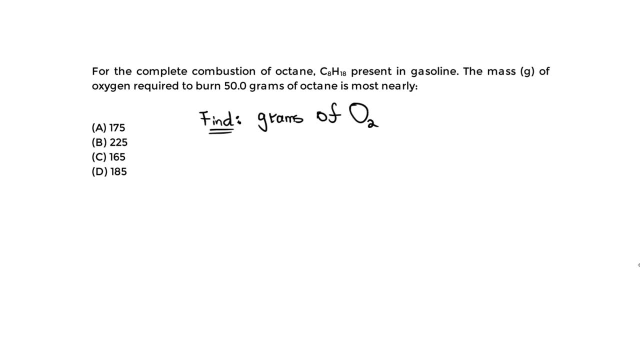 of oxygen, Let's call it O2.. So the grams of oxygen we need to completely burn 50 grams of octane. So now we will jump into the solution and we will begin by writing our chemical equation for combustion, specifically for the complete combustion of octane in gasoline. So we know combustion reactions have a reactant side and a product side. On the reactant side we will have the octane, which is going to be our hydrocarbon. 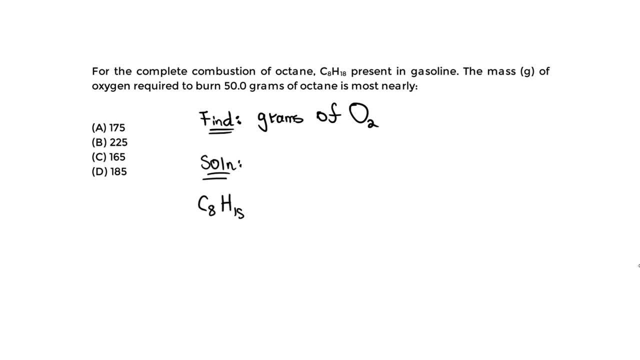 C8 and H18.. And we know on the left side, on the reactants, you have oxygen, right. So that's what's being mixed there On the left side, on the reactant side, you always have that oxygen. And just a hint there, that under combustion, in the environmental which is going to be on page 347 in the new FE handbook, you have a bunch of combustion equations and you see how in all of them it includes oxygen. 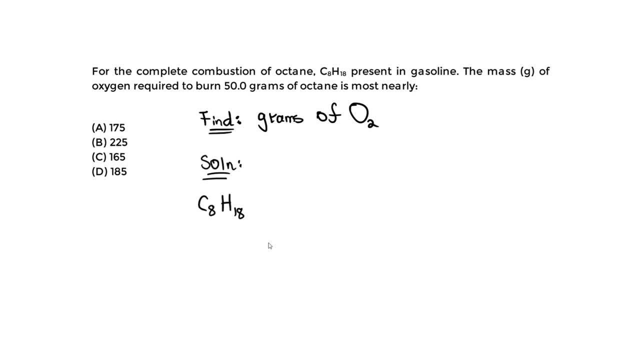 So that's going to be on the left side, right On the reactive side, So it's going to be the octane plus the oxygen And on the product side, the right side. what do we have? We're going to always have CO2 and H2O if we have complete combustion. If you have complete combustion, you always have what CO2 and H2O. So CO2 plus H2O. If you have incomplete combustion, you always have CO2 and H2O. 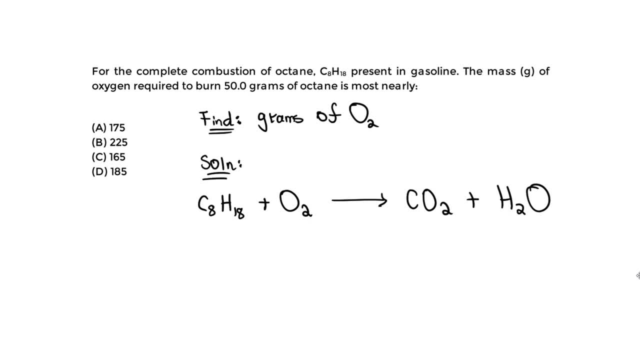 You might have other things. You might have some CO, which is carbon monoxide, which is actually toxic. So that's the difference there. When you have complete combustion, you only have these two all the time. So now let's balance this thing. 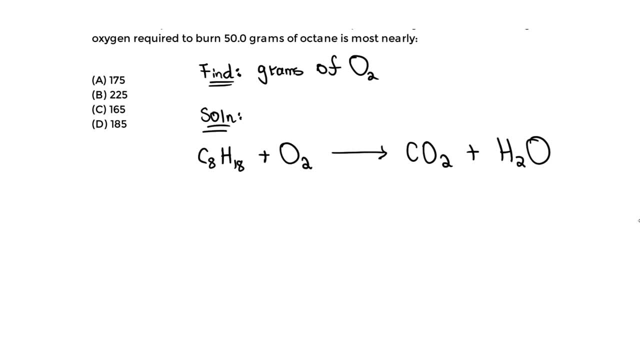 The first one is going to focus on the carbon. So how many carbons do we have on the left side? And let's compare that to the right side. On the left side we have eight of the carbons right, And on the right side we only have one. 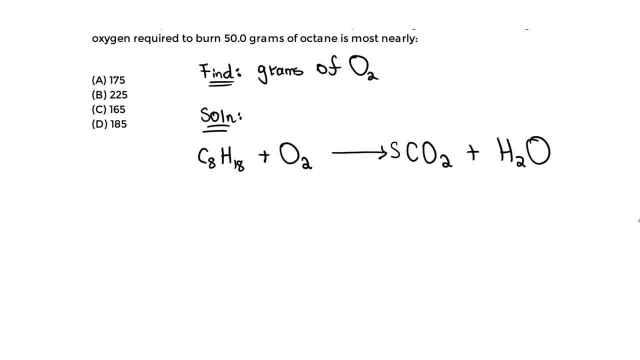 So we only have one here. So what we will simply do is place an eight here, Because we have eight. we place an eight here And we have eight of carbons now, So the carbons is balanced. Now we move on to the next one is the hydrogen. 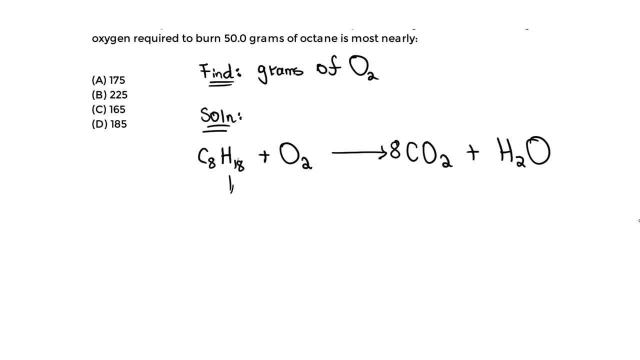 Next one is hydrogen On the left side. we have 18.. So we have 18 of the hydrogen right On the right side. how many hydrogens do we have Here? you only have two right. You only have two here. 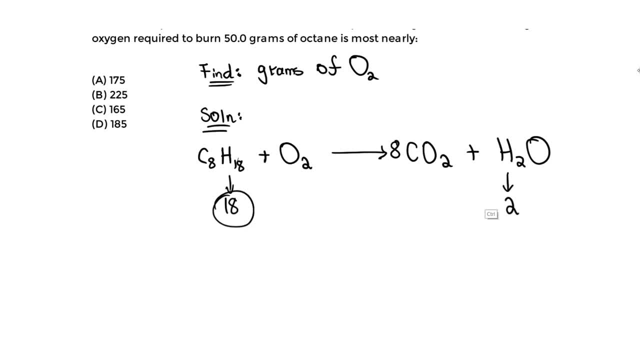 Two, Two, Two, Two. So we need this is bigger. The left side, the reactant side, is bigger than this, But we know we can multiply two by a number to get 18, right, What goes into two gives us 18?. 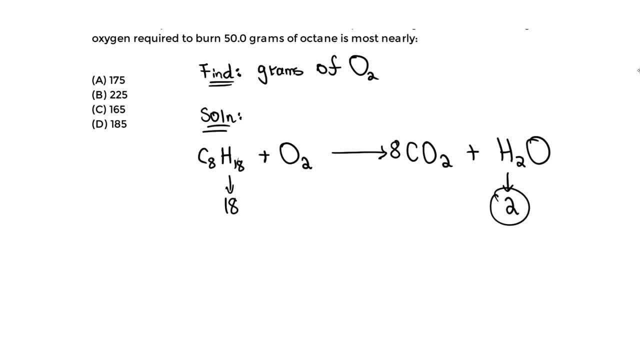 It's going to be nine. All we do is take 18 divided by two and we get nine. So here we can simply place a nine Nine times two gives us a new number, which is going to be 18.. So we have 18 here. 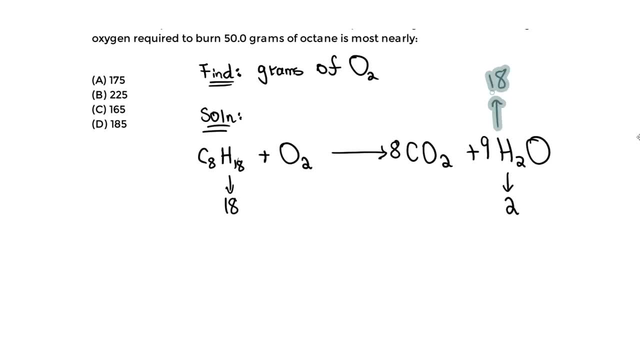 We have 18.. So the hydrogens are balanced, And now we will do the last one, which is always going to be the oxygen. So, on the left side, how many oxygens do we have? We have two, And on the right side, how many do we have? 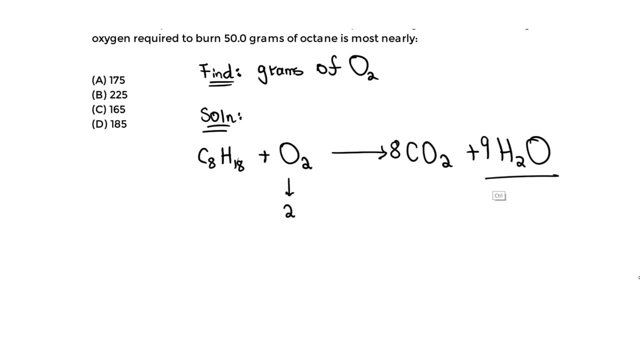 So here we have some oxygen, and so do we have here. We have both here and here. So here for the oxygen. eight times two is going to be what 16.. So that's 16 oxygen, Then plus nine times. 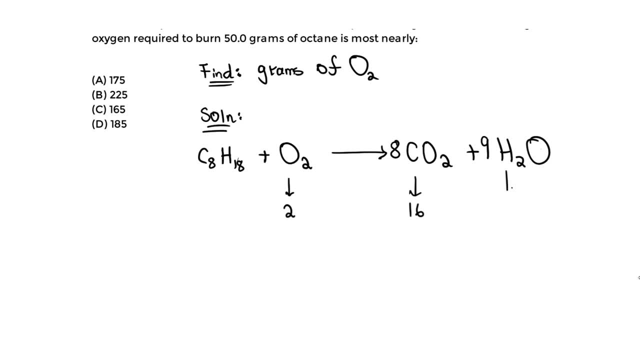 One. This is like nine of oxygen. It's just nine here right. So we have nine. So 16 plus nine gives us a total of oxygen of 25.. So now, on the right side, we have 25 of oxygen. 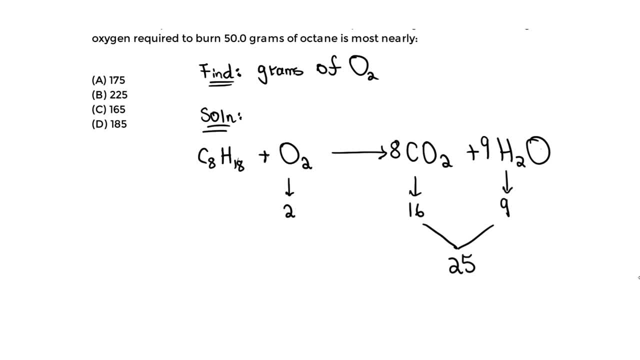 On the left side, we only have two. You do the exact same thing. We take the 25 divided by two and we can completely balance the left side to the right side. All we do is take 25.. 25 divided by two and that gives us a decimal value which we can get rid of, which is 12.5.. 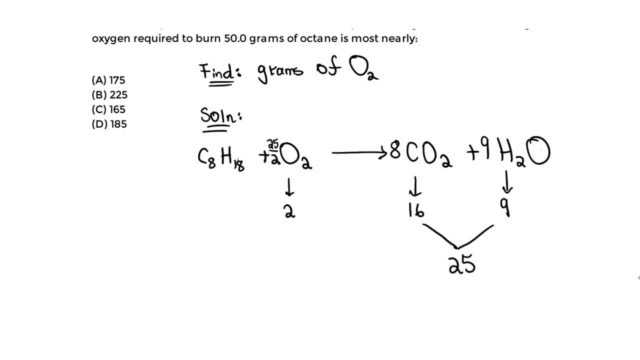 So 12.5 times two gives us 25, right, 12.5 times two gives us 25.. So now it's actually balanced. So let me erase all of this and this is how it should look like, and everything is balanced. 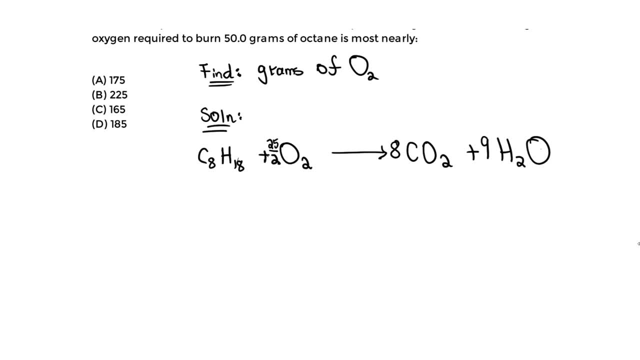 if you do a final check, All right, But what I'd like to do is simplify this further. if you want to, You don't have to do it, but you can simplify this further and get rid of this fraction, because we don't like seeing these fractions. 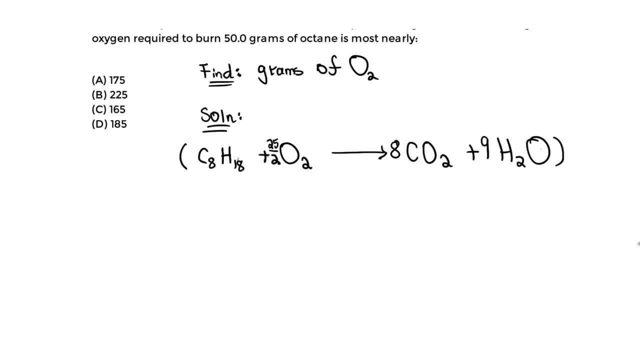 What you can do is multiply the whole equation. by what value? By two. So if I multiply the whole equation by two- which is what's on the bottom here- multiply that by two, You take two times this, So it's going to be 2C8H18.. 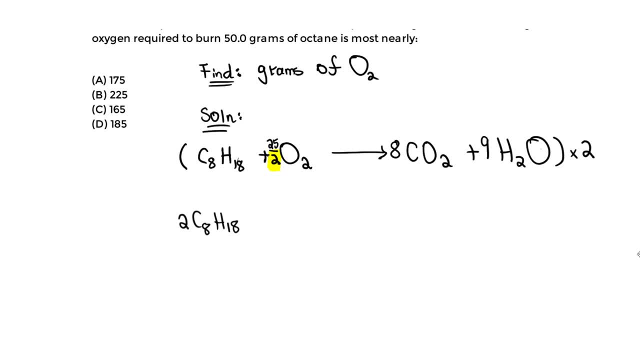 Okay, Okay. So you get 16 for the octane plus you take 25 over two times two, So 25, let me write that here: over two times two gives us what These cancel. It just gives us 25.. 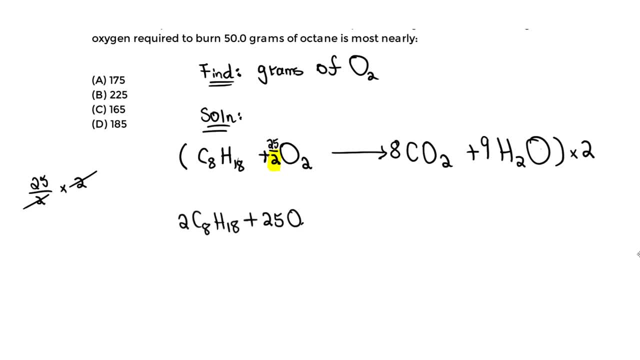 So we just get this here as the front coefficient, Then that is going to equal to the product side. So you take two times eight, You just distribute and you get 16 CO2.. Then you get two times nine, which is 18.9.. 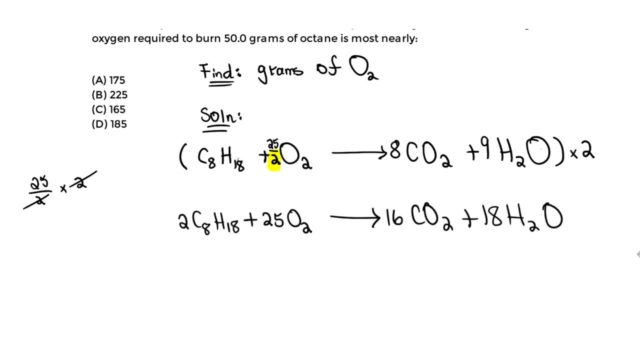 So it's 18.9.. 18.9. H2O- Okay, so you see how that looks neater and more so, all the coefficients are whole numbers, but again, you can just keep the fractions calm times and solve the question. 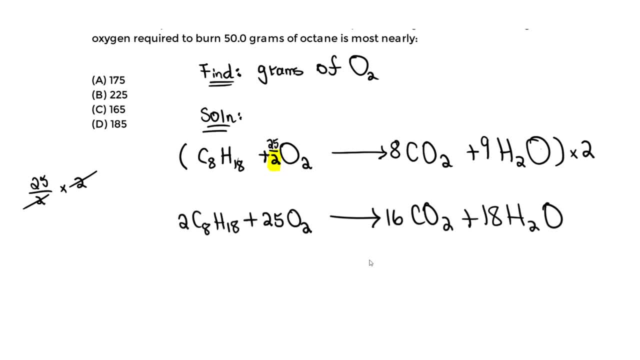 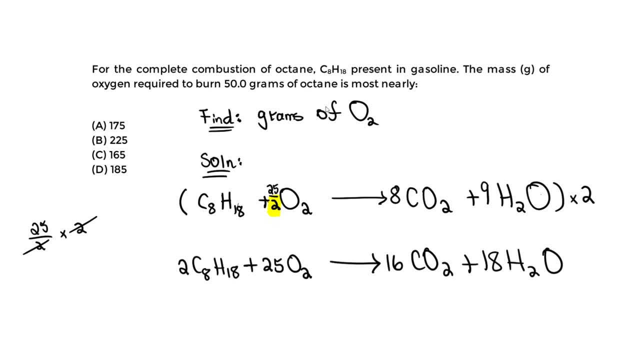 You don't have to do it this way, but this is how you reduce it to just whole numbers to eliminate the fraction. So now that's. the first step is to have the balanced chemical equation. Now we will actually solve the question. So we will start with the only value we're given. 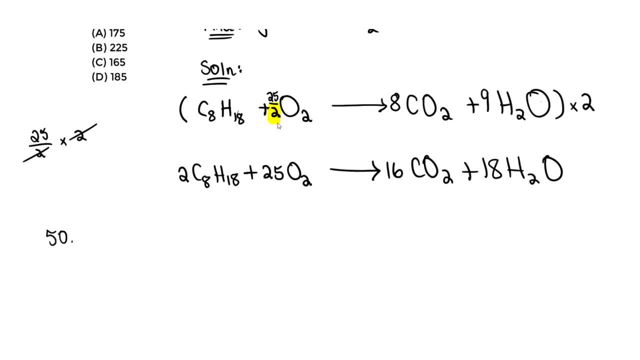 50.0 grams of octane. So we take that 50.0 grams of octane, which is CH18, that's what we start with and we know we're going to do stoichiometry, But before that we know. 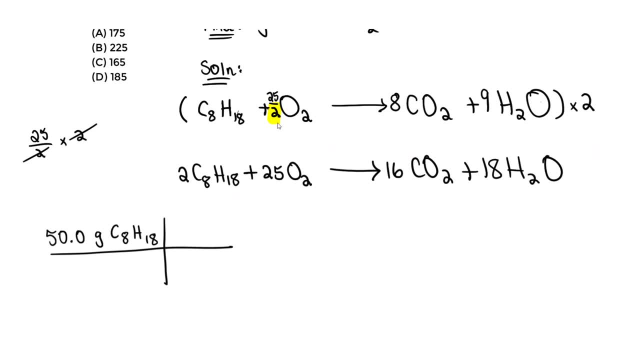 this chemical equation, the combustion equation, relates mole to mole. right For every 2 moles of octane we need to have 25 moles of O2 for a complete combustion, And we will use this equation when we do our stoichiometry analysis. So now we're like: okay, you have grams of. 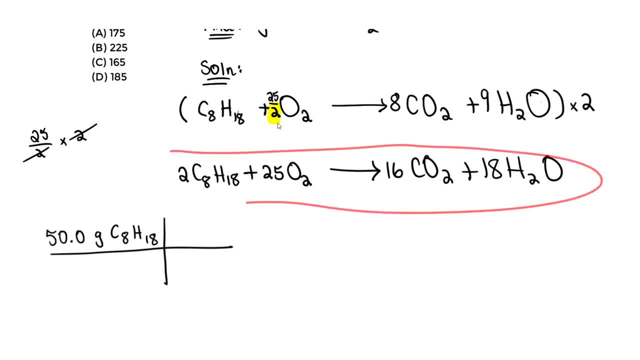 octane. how can I get moles? Because we want to use the equation to relate the mole to mole ratios. So we need to go from grams to moles and we have to use what We have to use the molar mass right. We have to take into account the molar mass of octane in this. 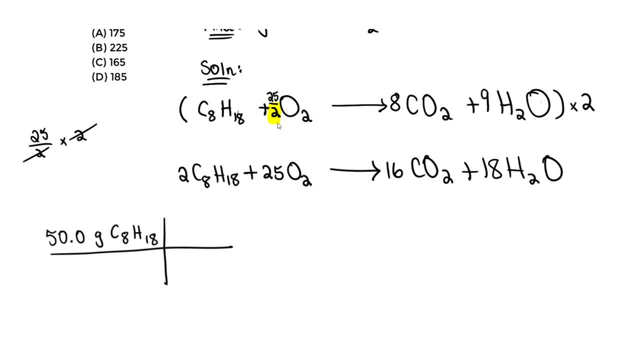 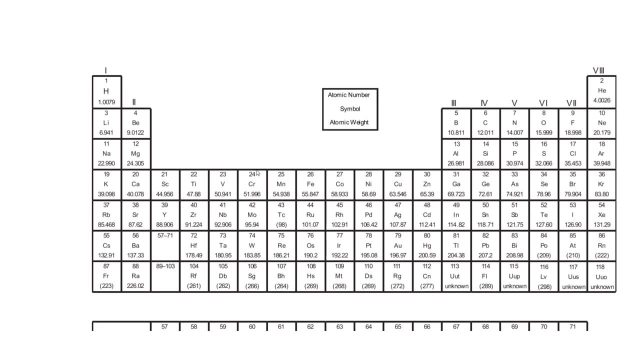 case, which has units of grams per mole. So how can you get the molar mass of octane CH18.. You just use the periodic table right. So you should have one in the chemistry section in the FE handbook. So for octane, we know we take C, which is going to be the 12th. 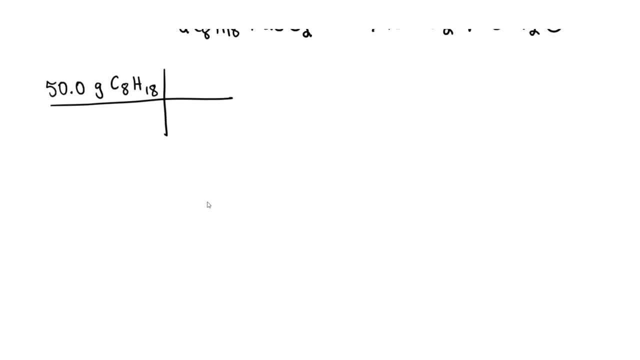 and we have 8 of that. so you do 8 times 12.. So let's do that here. Let me write the molecular weight of octane, which is the same as the molar mass. Do that. you take C of 8, so you have 8 of the carbon, right? So 8 of the carbon which? 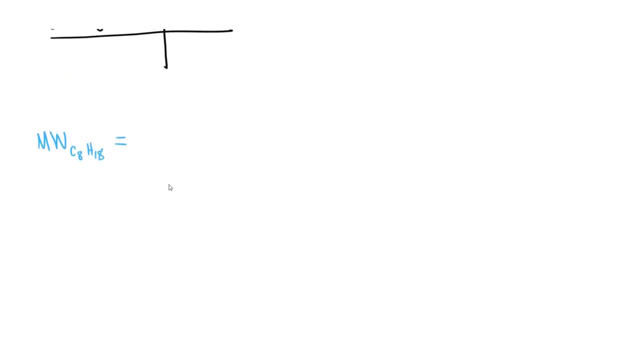 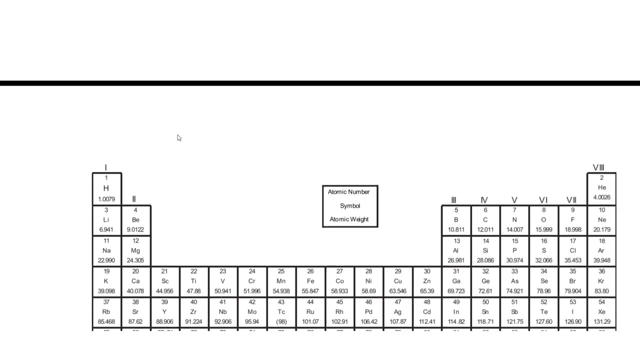 has the atomic weight of 12.. So you do 8 times 12.. 8 times 12.. Then you do plus, you have 18 of hydrogen, and hydrogen just has the atomic weight of 1.. The atomic weight is 1. 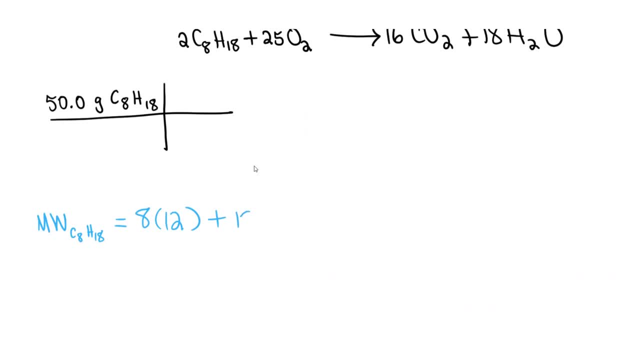 for hydrogen. So you just do 18 times 1.. And if you do that, let me do the math. you do 6,, 18, and you get about 114.. And note the units are what It's going to be: grams per. 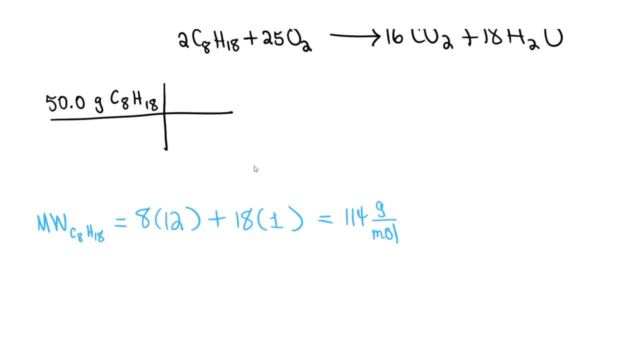 mole. Grams per mole, That's going to be the units for the molecular weight. So what we can do here is say we know grams is here. what's up here must come down here, right, So the units can cancel It has to. what's up here must come down here, So we know we. 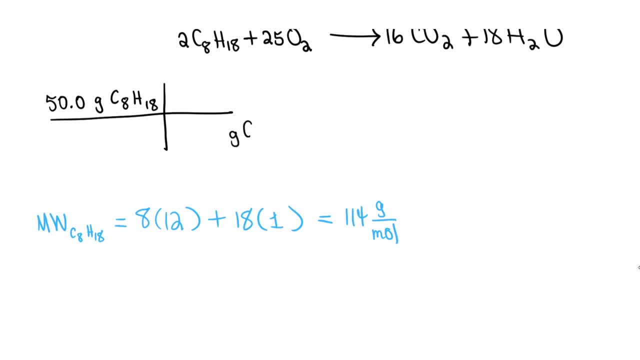 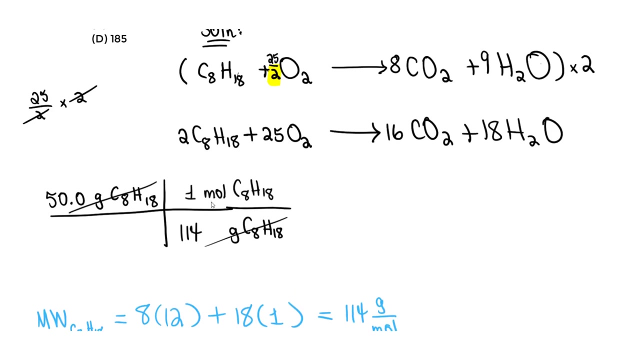 will put C- sorry G- the grams CH18. And we know that's going to be grams, so it's going to be 114 grams per 1 mole of CH18.. So now these cancel right. So now we finally got it into moles, So we have moles, and when? 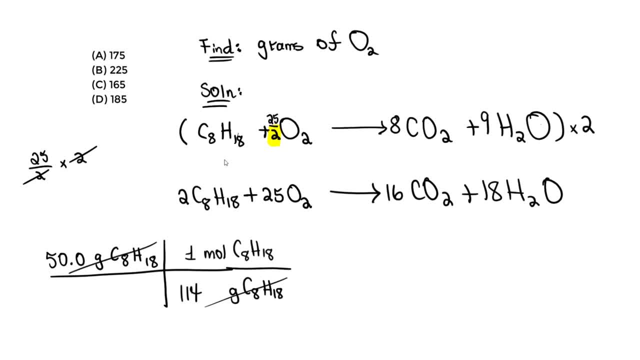 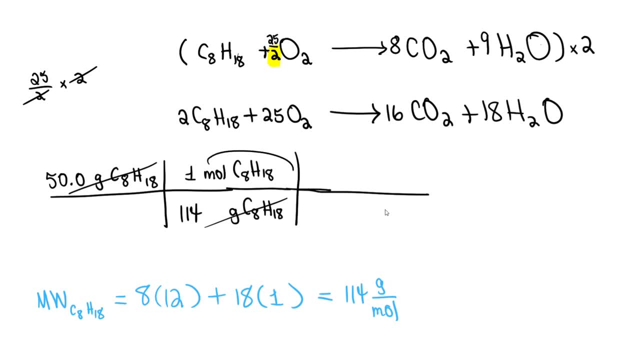 we have moles here. we can also use this chemical equation and relate the mole to mole ratio. So with the chemical equation above we know, here we have moles, so it must come down here: moles of CH18.. And now we know we need 2 moles. 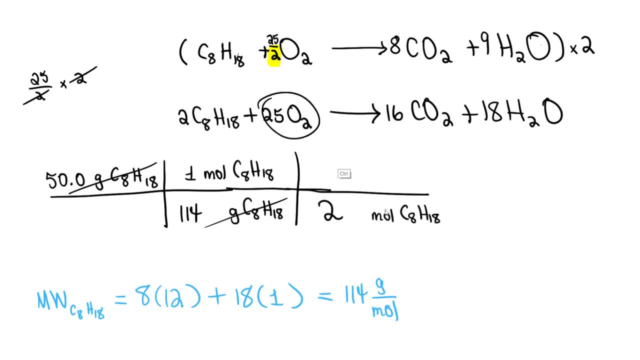 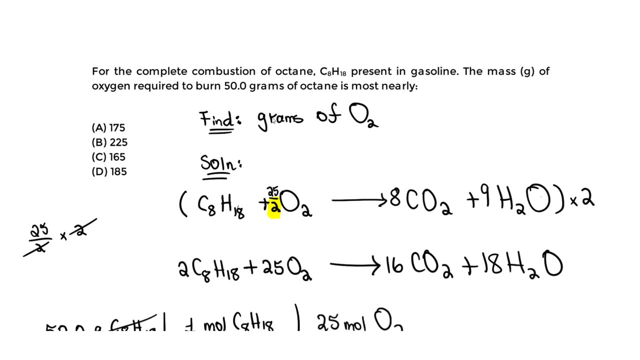 of CH18 for every 25 moles of oxygen. 25 moles of oxygen. And you might ask: okay, why did you choose moles of oxygen? Because that's what we want to find right, We want to find the grams of oxygen which we will get to. We're comparing the octane to oxygen. 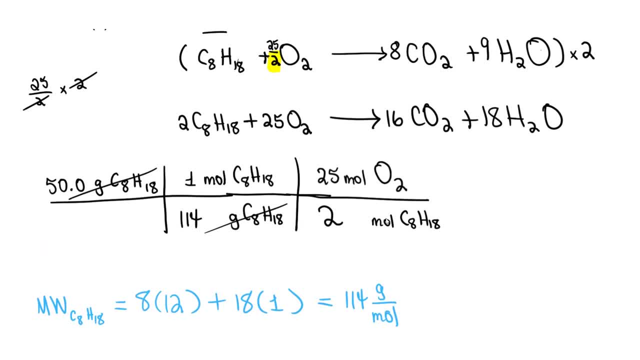 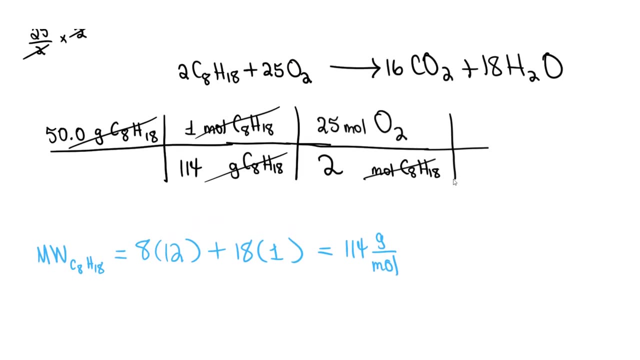 So we're going to compare the mole to mole ratio of octane to oxygen. So we know these cancel. So we're almost done. Now we have moles of oxygen But we need to do what We need to get grams of oxygen. And how can we do that? You use the molecular weight for 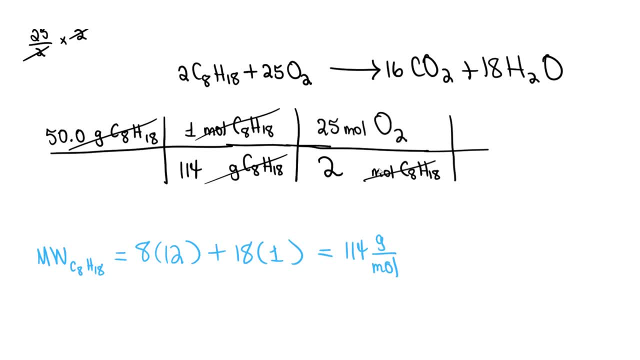 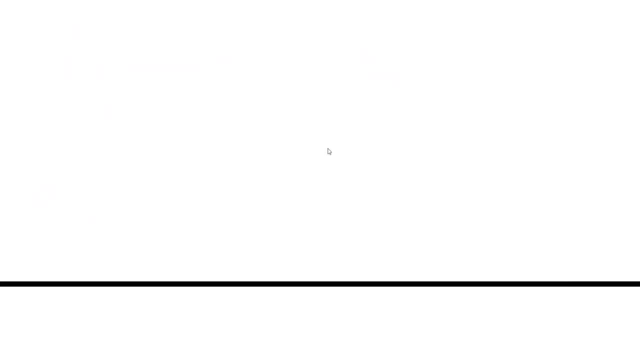 oxygen. But we have, we know we have- 2 of the oxygen. So the molecular weight of oxygen. look at the weight of O2, equals. let's go down here For O2, where's oxygen? It's this: 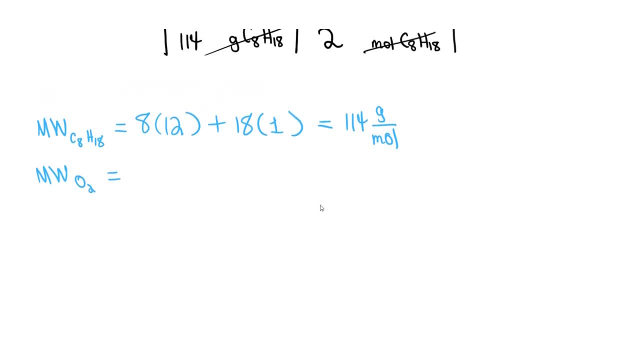 right, 15.999.. So it's about 16.. So you do 2 times 16.. 2 times 16. And we get 32.. So this has units again of grams per mole, And this is for oxygen. We have 2. So you multiply. 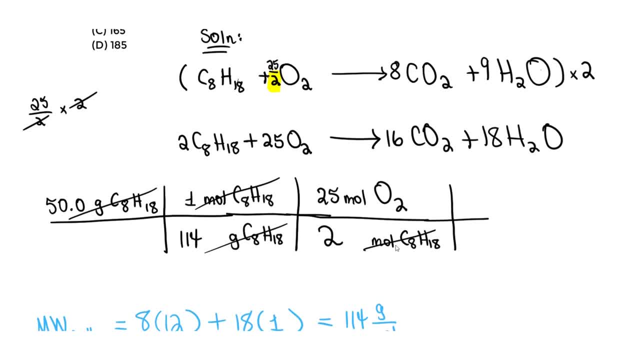 2 times the atomic weight of 16.. Get 32.. So now what we will write is: we know for every 1 mole of O2, which is this right? It can be this, and it must come down here. So for 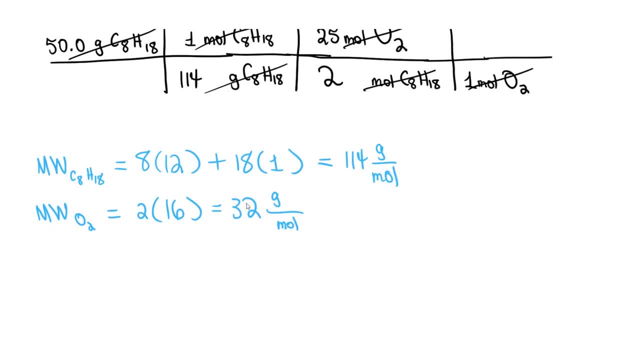 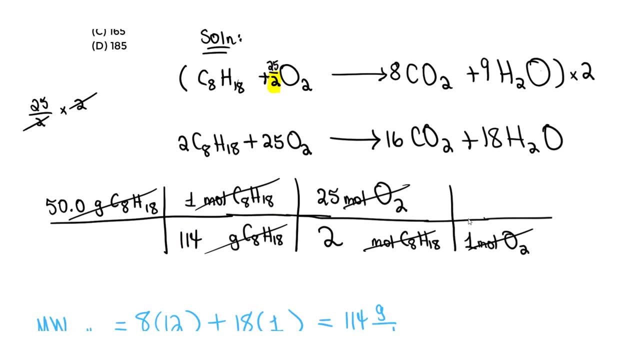 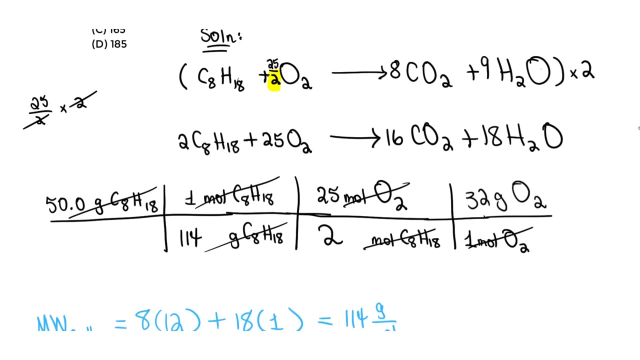 every 1 mole of O2, these cancel. We will have 32 grams of O2, right, 1 is on the bottom, 32 is on top. You have 32 grams of O2.. And notice how everything canceled and the final. 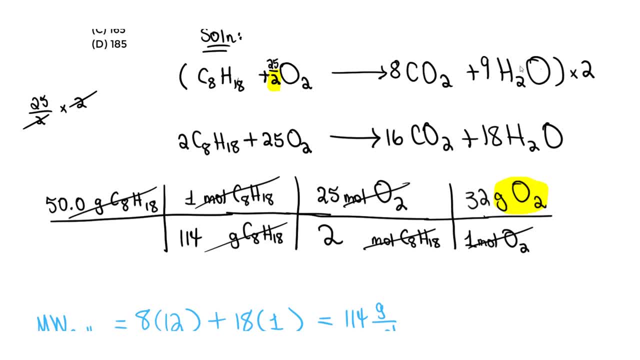 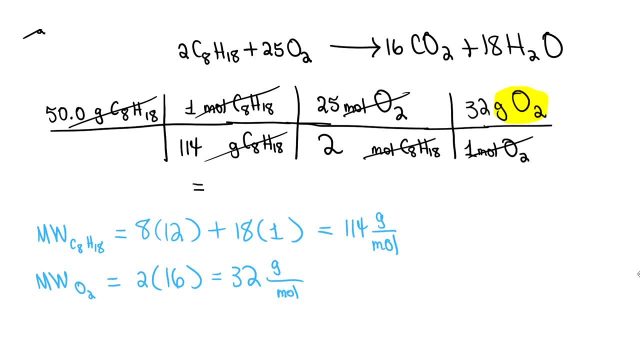 units are grams of O2.. And that's going to be what we do, right? That's going to be the answer, And you just do the whole math for that. You do the top portion divided by the bottom portion, And I believe we should get around 175.44 grams of O2.. So here, this should be our answer. 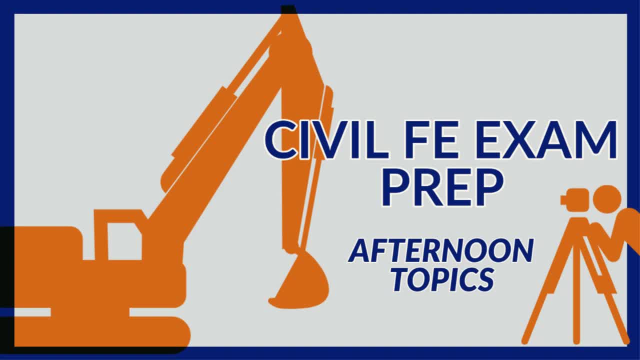 And in this case it should be A. So, to finish off this video, I want to introduce, and I'm excited to announce, my new Sibyl FV prep kit. Sibyl FV prep course for the afternoon topics on the Sibyl FV exam. So I've been working. 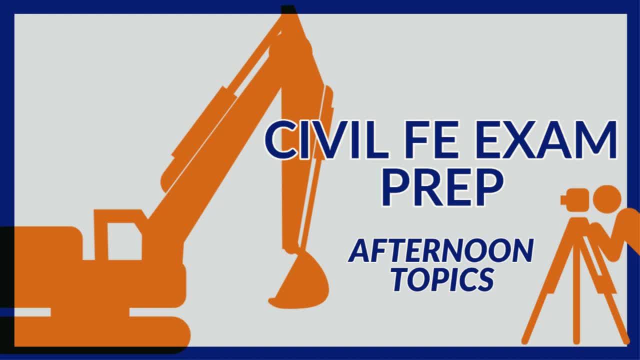 on this course for some time now and I feel like it's finally time that it's released to help you pass the Sibyl FV exam. So we cover all the concepts, all the topics, with hundreds and hundreds of practice videos. 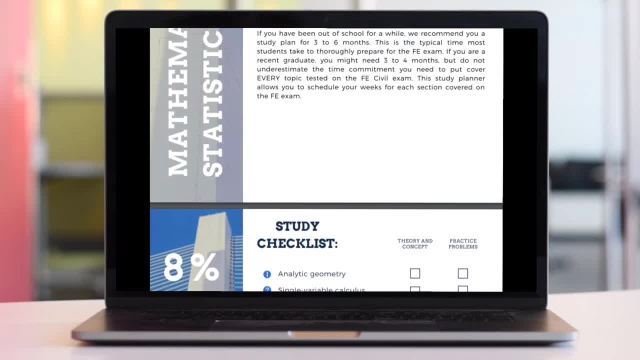 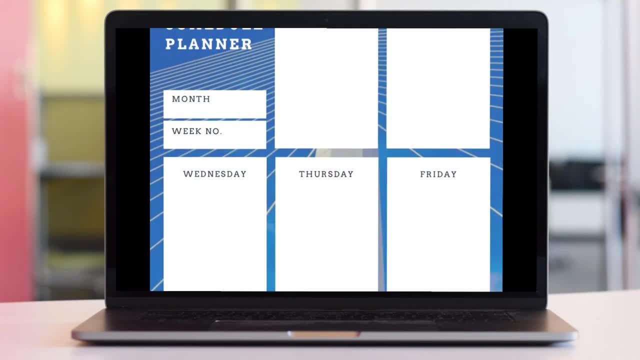 So if we look at some of the course features, you will get a total, complete PDF study planner. So this is made specifically for the Sibyl FV exam with an equation sheet, with the weekly plan, a checklist, some exam tips, areas to improve section and the big wins. 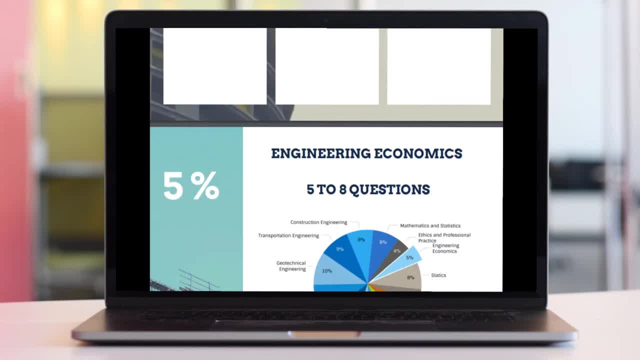 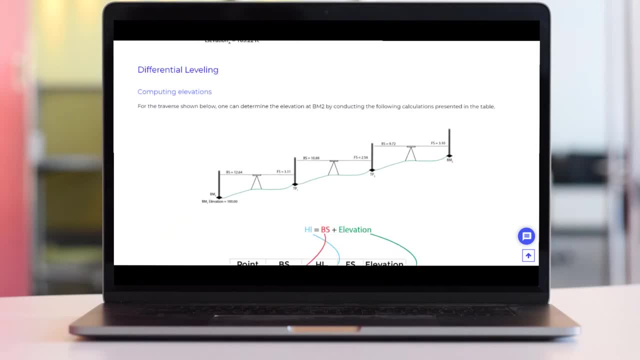 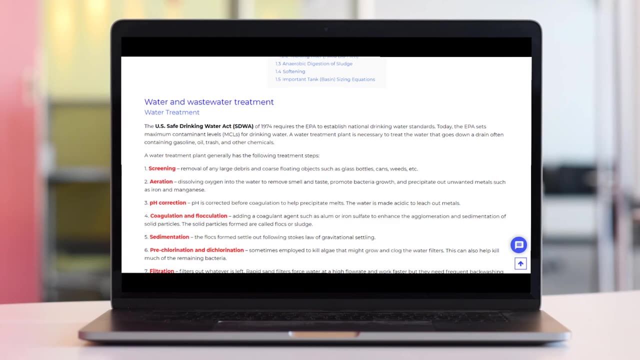 section. Again, this is specific to the Sibyl FV exam that you will get with this course. Next, you will get 50,000 plus words of lesson notes that reference all the topics and equations you need to know for the Sibyl FV exam. So these lesson notes come with full figures. 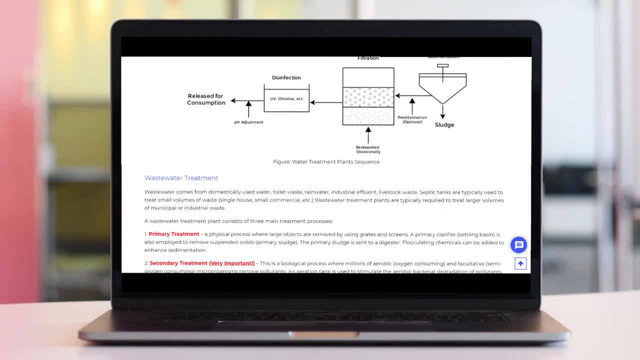 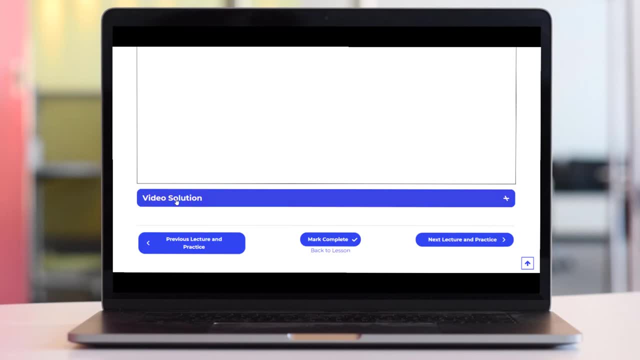 full, simple explanations, and everything is built from scratch specifically for the Sibyl FV exam. Now for the most important part: you will have access to hundreds of practice questions with full video solutions where I walk you through the step-by-step procedure needed. 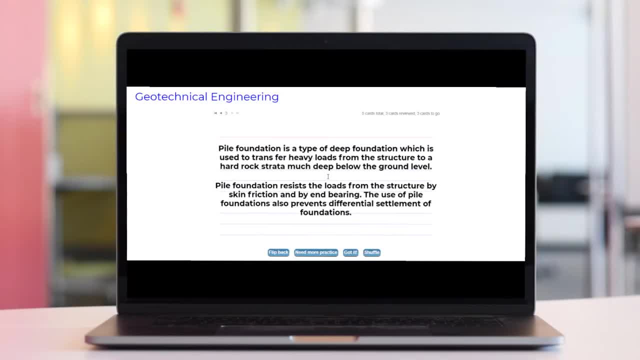 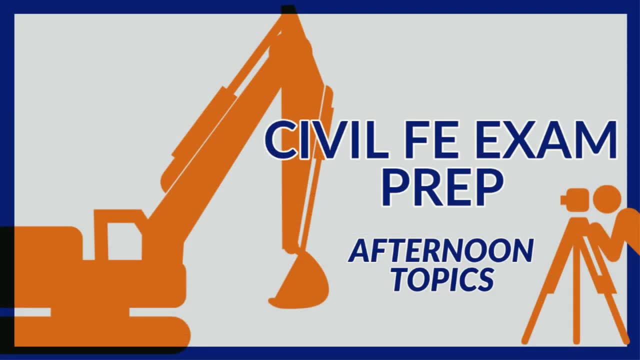 to solve each question. And, lastly, you will have access to hundreds of flash cards that are guaranteed to help you answer those conceptual questions on the Sibyl FV exam. So, on top of all these course features, you will have complete access to me when you have. 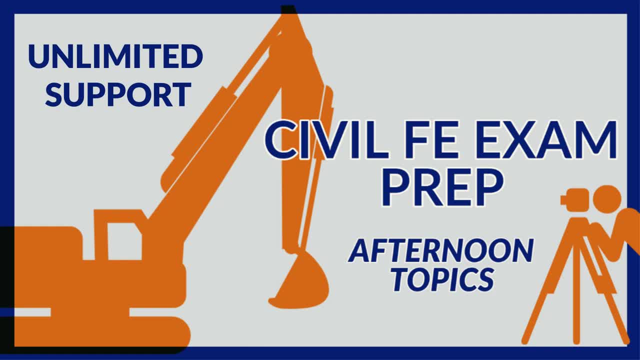 questions. get stuck on a question: need help setting up a course, or when you need help setting up a course, or when you need help setting up a course, So I will be sure to up a schedule plan and a steady schedule, or just need that extra guidance to help you. 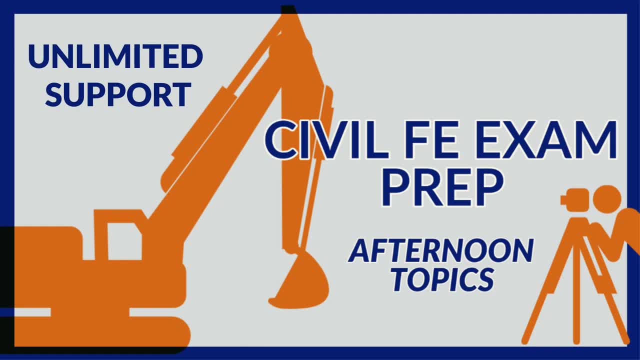 stay on track. To learn more about this course, please check out the link in the description below and if you have any questions at all, you can email me directly at Farouk at directhubnet. again, that's Farouk at directhubnet.